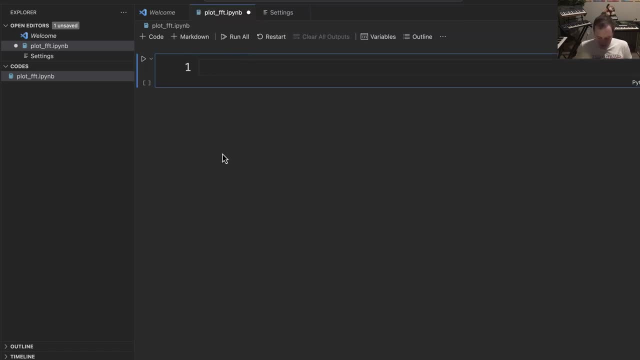 VS code, like I am, it'll automatically find it for you. So what I'm going to do is import numpy as np, and we want to import matplotlibpyplot as plt, so we can actually plot things. So now what I'm going to do is define xfp. 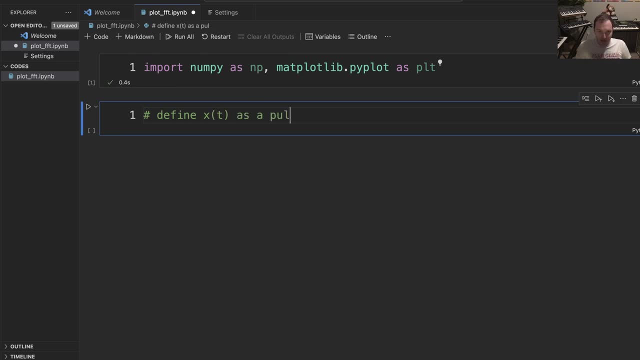 As a pulse function. So what I'm going to do is say num- t equals 100, and we're going to say xt equals numpyzeros. So we're going to have a bunch of zeros, and I want to have 100 of them. 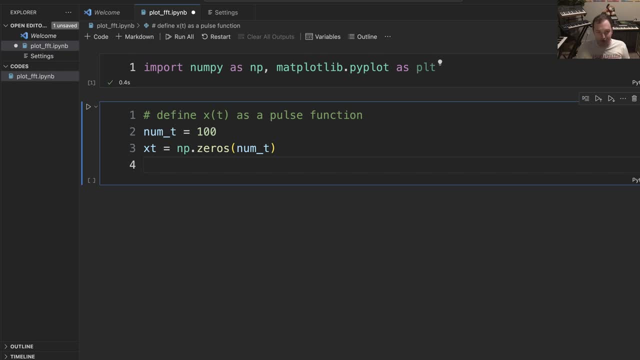 So I'm going to put that in there and what I'm going to do next is just say xt from zero to up to nine. So it's not inclusive of this second number. So it's going to be zero one, two. 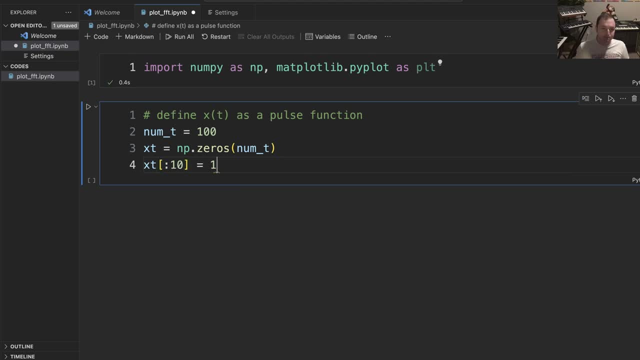 three, four, five, six, seven, eight, nine, not to 10.. I'm going to say xt equals one, and what we're then going to do is now, I'm just going to plot the signal. So that's why we imported matplotlibpyplot. We're going to just do pltplot x of t and 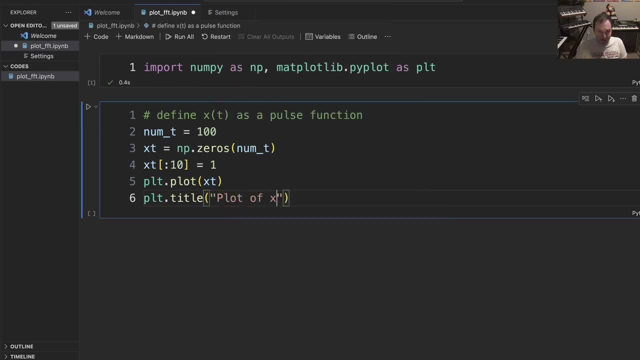 I'm just going to give it a title: plot of x of t- xlabel Now, because we don't have an actual xlabel here. this is just going to be the sample index and pltylabel is going to be the value of X of T. So let's go ahead and plot that And, sure enough, what we see here is this pulse, or 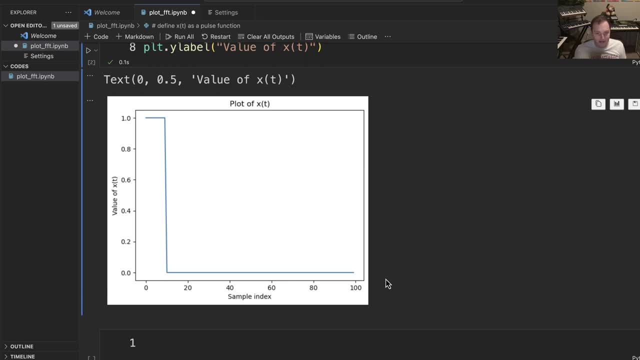 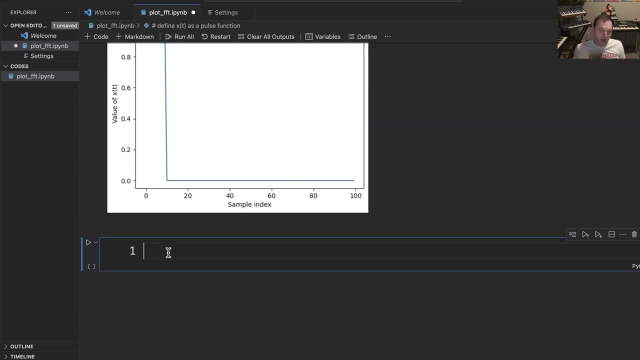 this box function all the way up to nine and then it flattens out and it's zero otherwise. So we defined it as zero and then we just basically set these guys to be one. Now let's go ahead and plot the Fourier transform of this, or the FFT. So the way to do that is, I'm going to say: 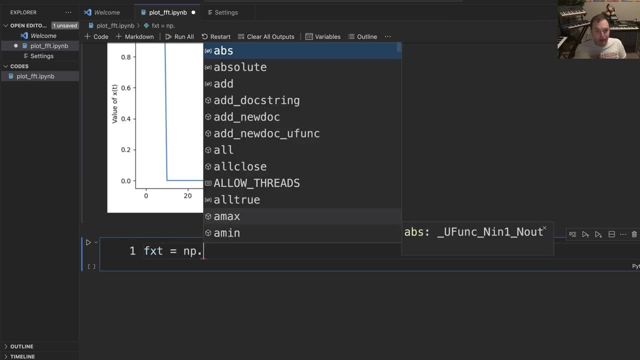 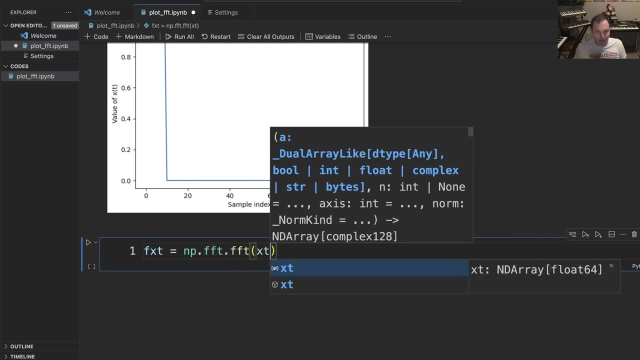 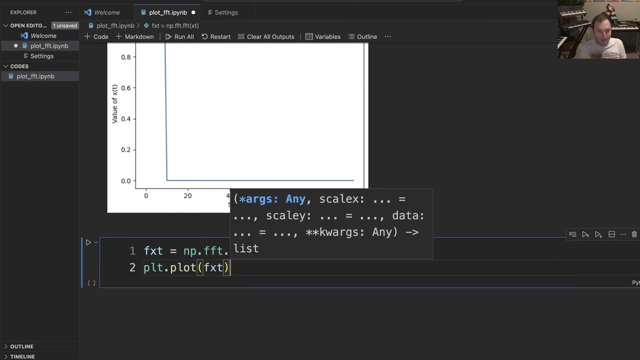 FXT equals numpyfftfft. So we're calling the FFT package and we're just calling the simple FFT function and we're going to pass in X of T. So now we have this, we can go ahead and plot it. So I'm going to say PLTplot, FXT. PLTtitle, plot of FT of X of T- PLTyLabel. 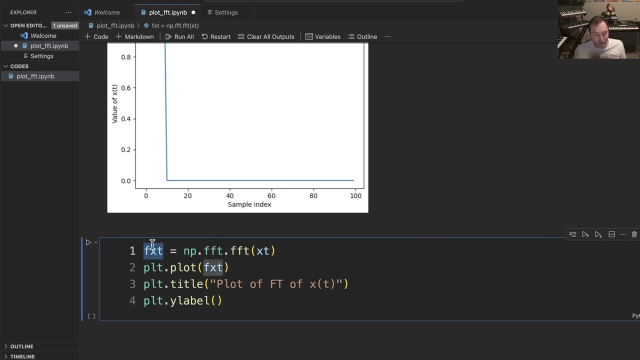 Now, this is difficult because remember that the Fourier transform is going to have both real and imaginary parts, And that's one thing that's really important to realize is that you actually are going to have two plots: one for the real and one for the imaginary. 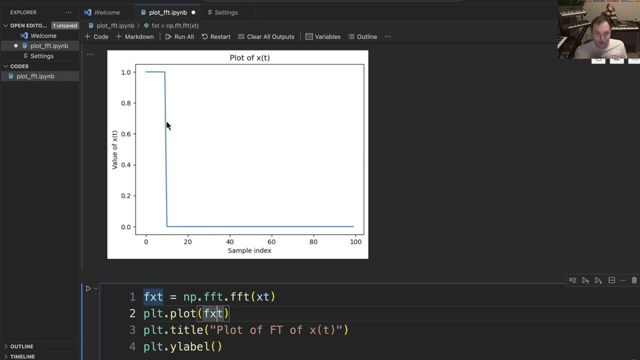 Now what some people always ask is: well, I'm putting in a real signal, Shouldn't I only have a real Fourier transform? The answer is no, And that's because, remember, you have even and odd parts whenever you have any signal and all of the even parts get shoved into the cosine term or the 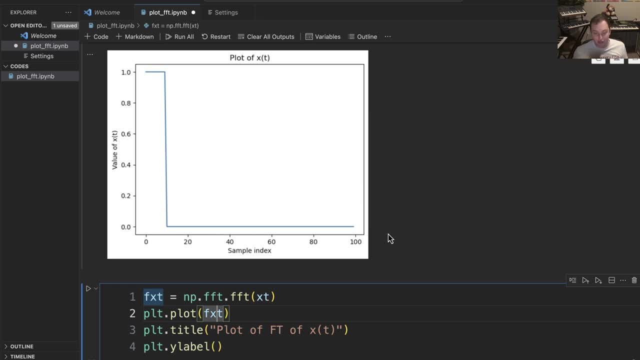 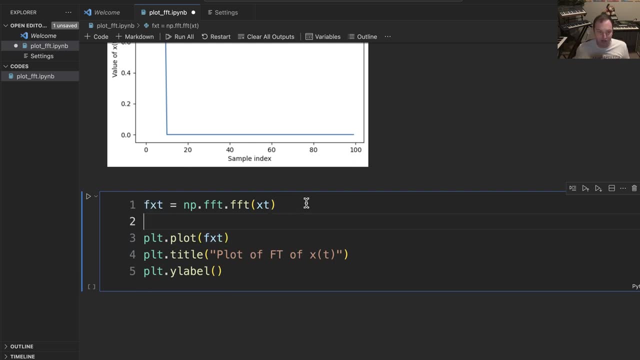 real term and all the odd parts get shoved into the sine term, which is purely imaginary. So a signal that is both- you know that is not necessarily even or odd- is going to have real and imaginary parts. So let's go ahead and split this up into two different plots. 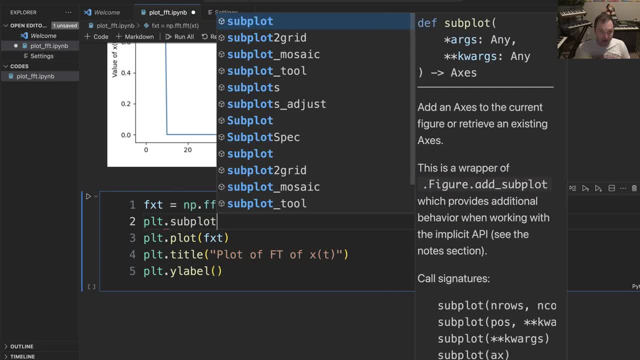 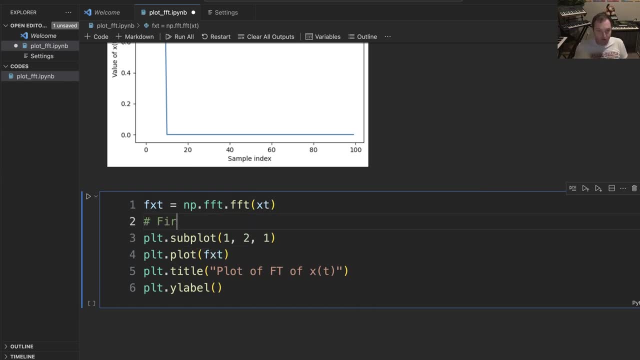 So the way I'm going to do this is, say, PLTsubplot, and I'm going to create a one by two grid of plots and this is going to be the first one. So first plot is the real part and we're going to PLTplot. 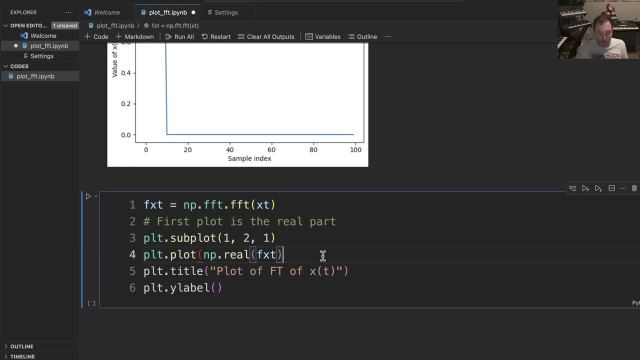 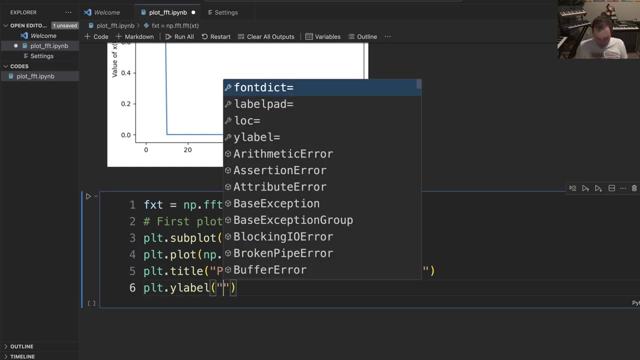 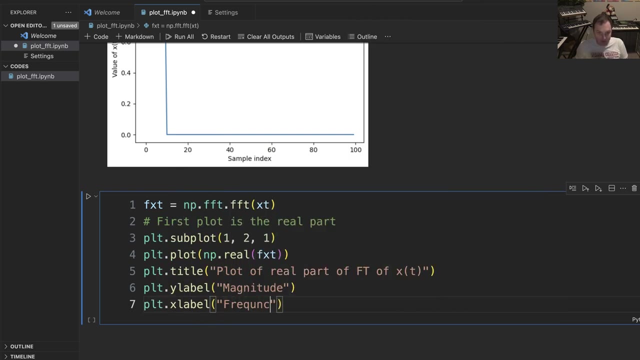 numpyreal, the real part of the Fourier transform, Fourier transform of X, of T. So the Y label is going to be the magnitude and the PLTxlabel The Y label is going to be the frequency index And similarly I'm going to do the imaginary part as well. 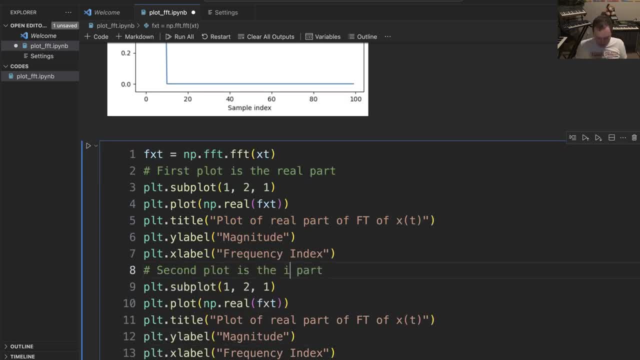 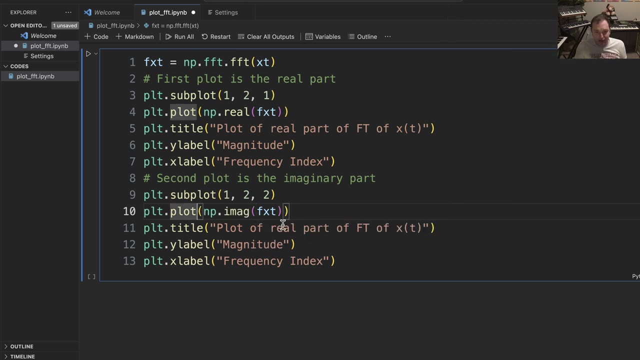 So this is the second part, which is the imaginary part. We need to look at the second subplot. So this controls the index. So it's a one by two. This is the first, I guess, plot and this is going to be the second one. So this is numpyimaginary and this is plot of the imaginary part of this. 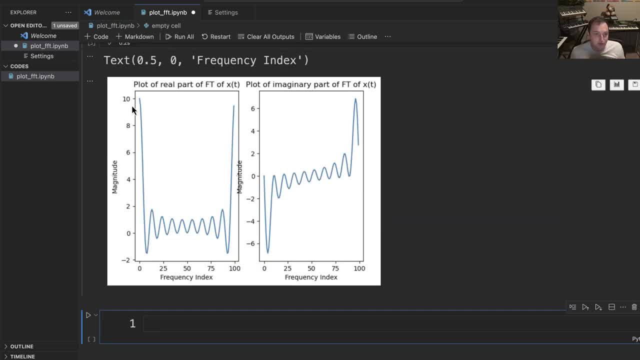 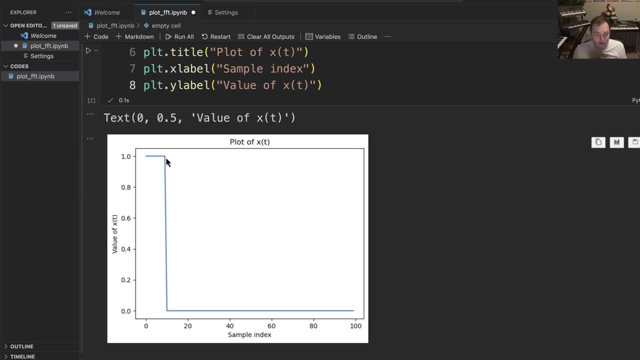 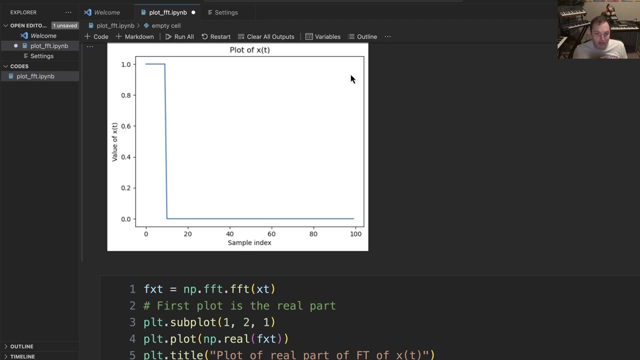 So, sure enough, I run this and what we see is we have both a real signal. this is the real part, and we have the imaginary part, because our signal here is neither completely even nor odd, It's a little bit of both. And by even is what I mean is X of T equals X of minus T, so it would 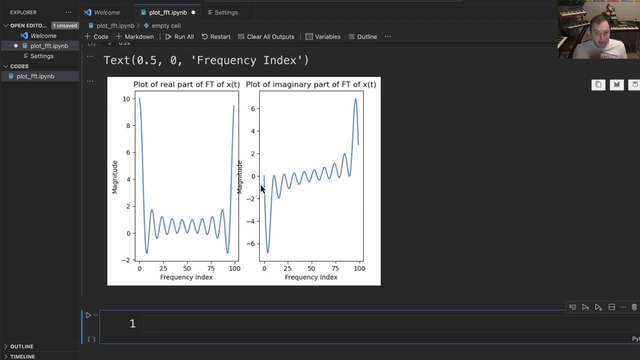 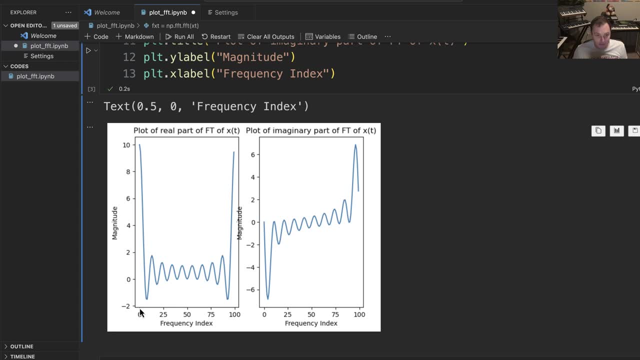 need to be mirrored across the middle here. Now, one thing that's a little bit confusing about the way this is plotted- and this just has to do with the way the transform itself is done- is we start at zero frequency, Then we go up? 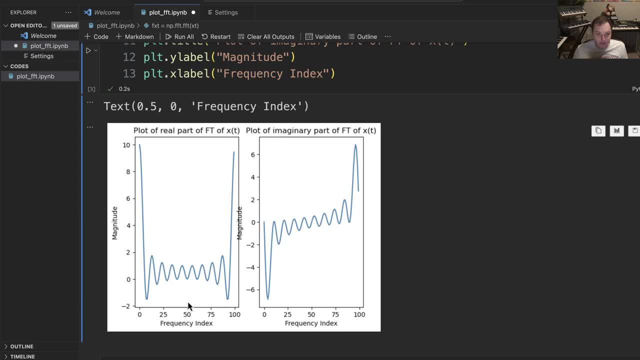 To halfway And then after halfway we then jump from the highest frequency we have to the lowest negative frequency we have. So we go up to, you know, basically, frequency index 50. And then now, at 51, we're now plotting frequency index of minus 50, pretty much. So this can be a little bit. 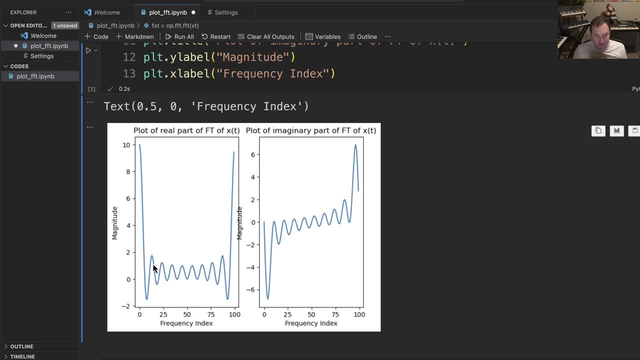 confusing because of the way that it's plotted. This doesn't look like our standard sync function that we're used to seeing. So there's this really nifty feature. It's present in MATLAB and it's present here in numpy, called FFT shift, And what that'll do is it'll take this: 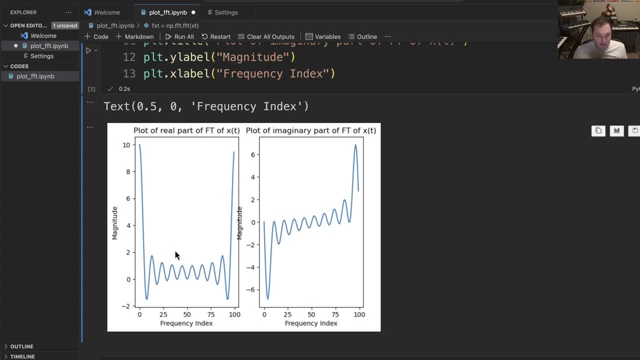 half of the frequency that we have and we're going to go up to the lowest negative frequency. we have Half of the signal and it'll just bring it over here and shift everything to the right. So that way you're looking at this: from left to right, You start with negative frequency, you have zero. 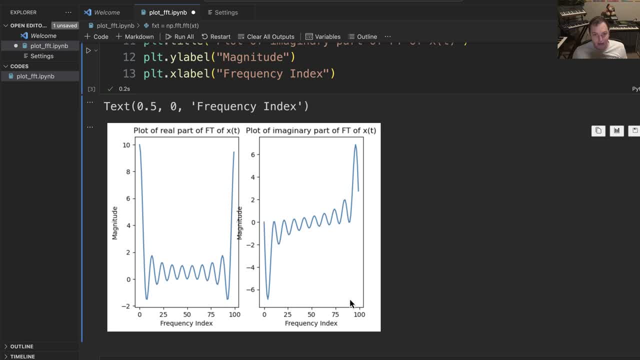 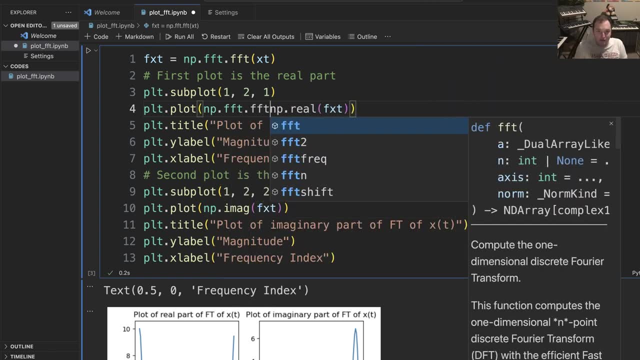 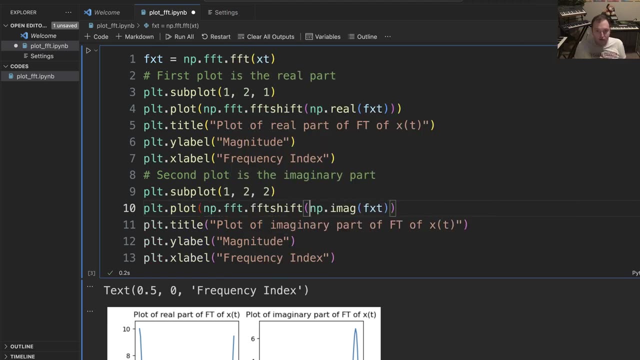 frequency in the middle and then you have your positive frequency on the right, Same with the imaginary part. So to do this, all we have to do is just type in numpy dot, FFT, dot, FFT, shift. And I'm going to do that over here, Like so. And sure enough, when I plot it, look we have. 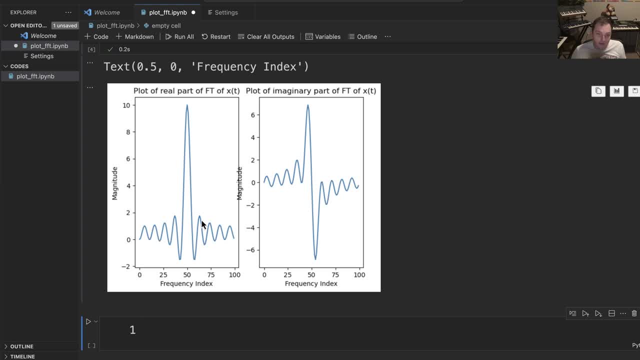 our standard sync function. It's completely real, Or sorry, it's completely. yeah, this is the real part and it's even as we expect. And then this is the sort of odd part here. This is what we see from the conjugate symmetry, The reason we see this, where the imaginary part, the positive imaginary, 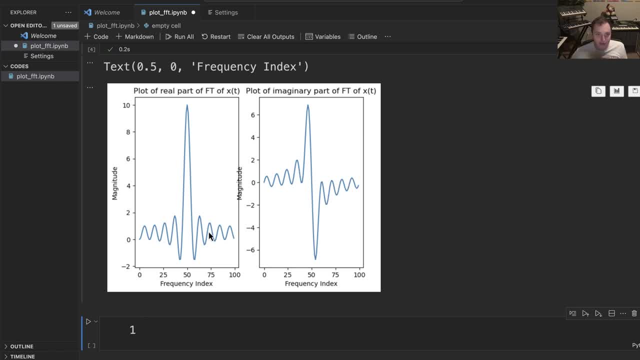 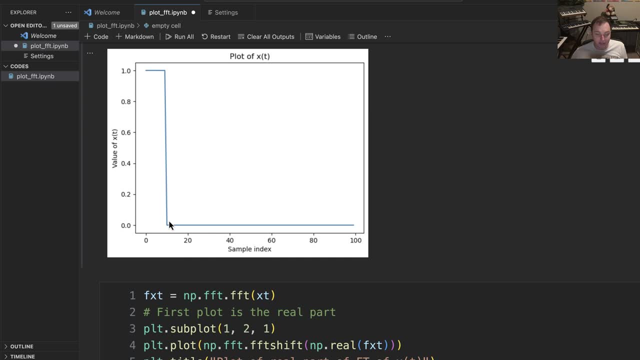 part is equal to the negative of the negative imaginary part. And then for the real parts, the real part is basically equal to the negative of the real part is because this signal was completely real and a real signal is going to have conjugate symmetry, meaning the real part is going to be: 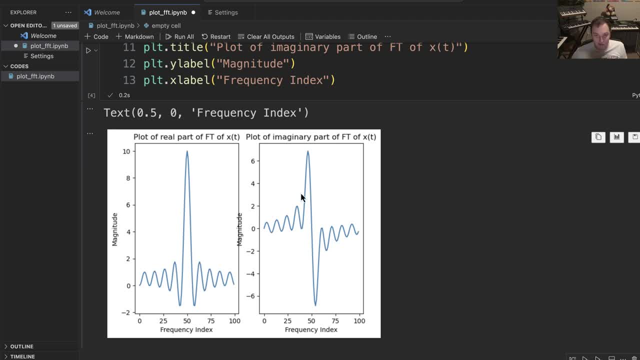 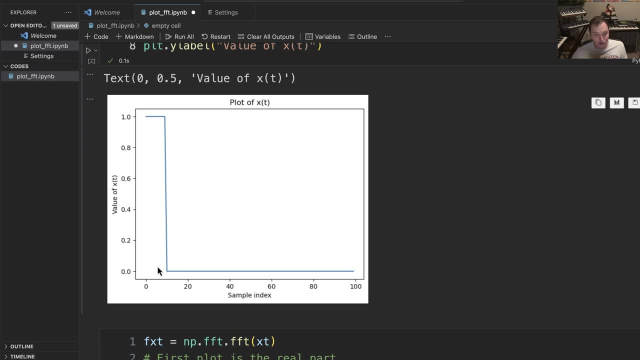 even symmetric and the odd part is going to be odd symmetric, which is what we see here. Now, what I want to do is show you what happens when we actually get an even symmetry in the time domain. Doing this the right way will actually cause us to only have a completely real Fourier. 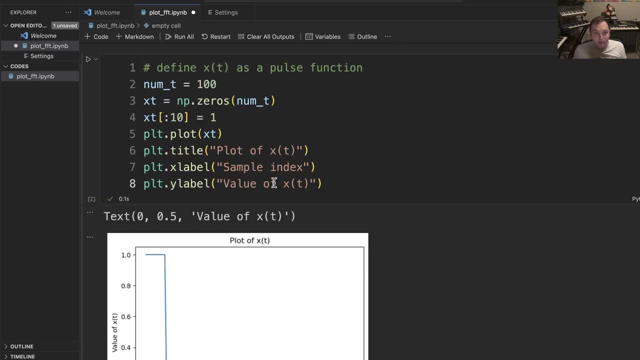 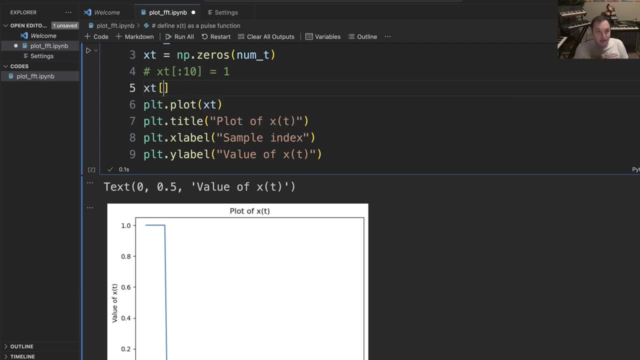 transform. There shouldn't be any imaginary part. So the way I'm going to do this is, rather than setting zero to nine to be equal to one, What I'm going to do is say xt from zero to five. So this is going to be zero one, two. 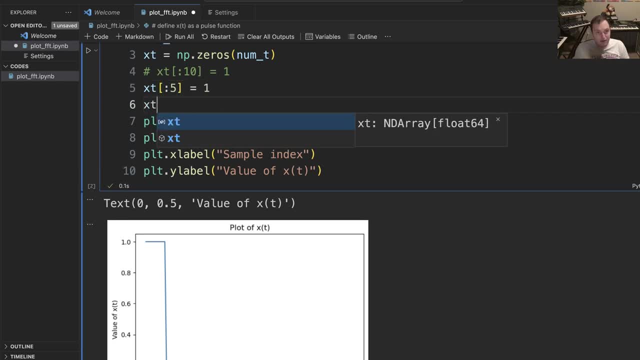 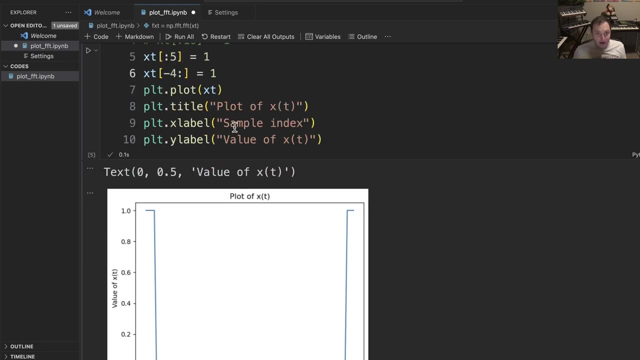 three and four is going to equal one. And then what I'm going to do is say xt, from minus four to the end, is going to be equal to one. Now, why am I doing this? What this is going to do is this is going to set zero, one, two, three and four, So these five elements to be one. And then why I? 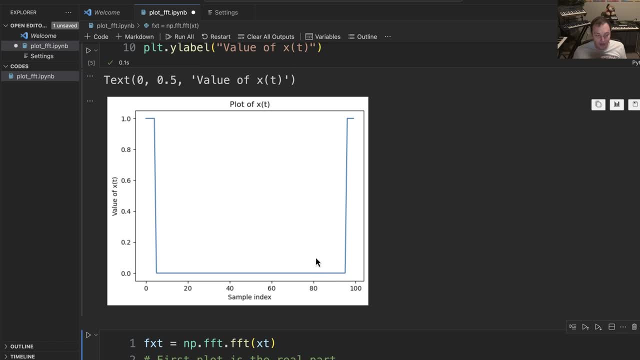 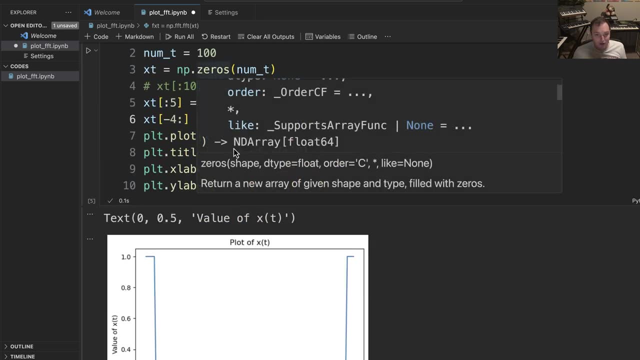 need to do minus four to the end is it's going to be the n minus four, the n minus three, the n minus one and then the very last component, equal to one as well. So this is going to ensure we have the symmetry that we need, And let's go ahead and see what happens when we plot it Sure enough. 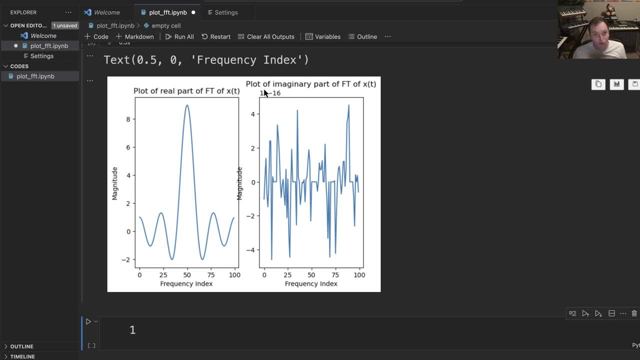 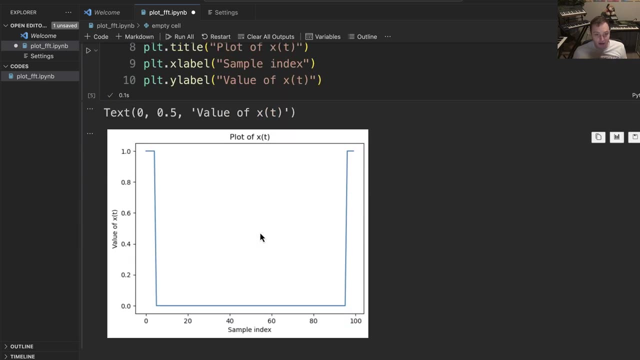 notice what we have. This is the imaginary part, and it's pretty much zero. This is one times 10 to the minus 16.. So that's pretty much down to numerical precision, And what we have here is a completely even signal as well. Now suppose our signal was completely odd. 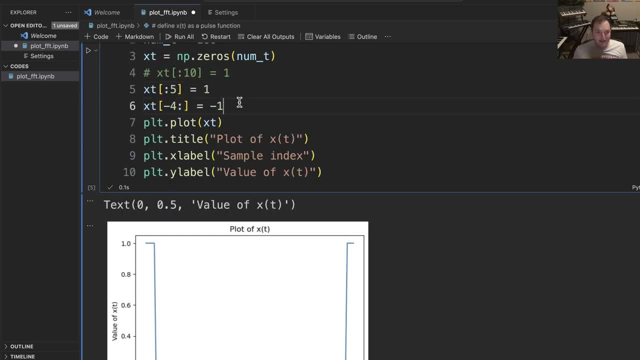 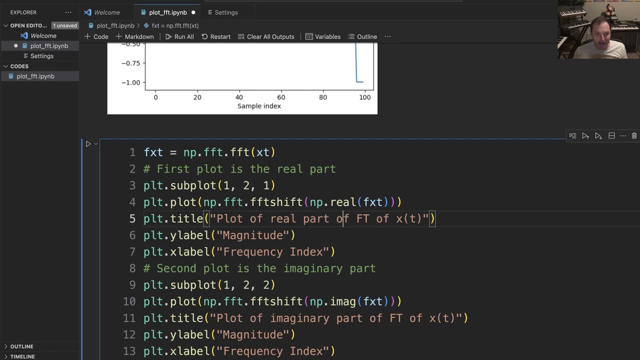 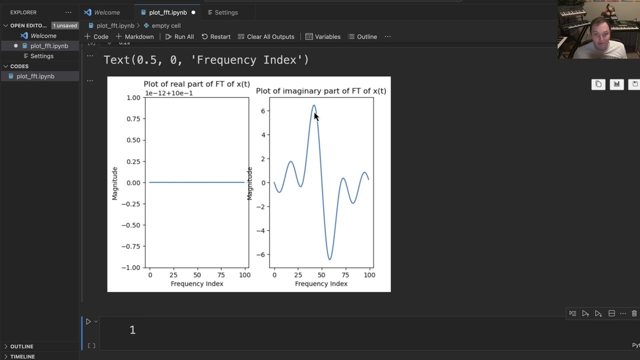 That would mean, rather than we had one here and then we had minus one down here. So if I plot this, this would sort of be like an odd type of signal. And if we look at the Fourier transform, sure enough this is what we have. We have zero for the real part and our spectrum is completely. 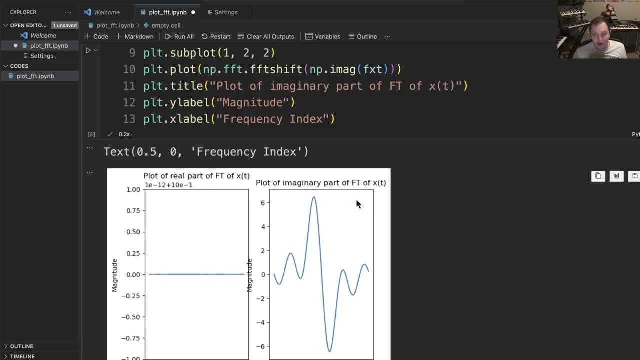 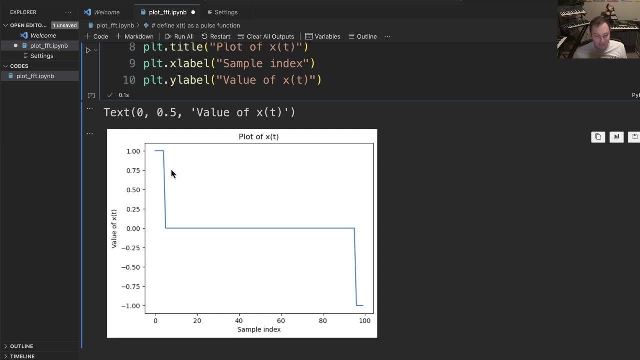 imaginary. So remember that distinction between even and odd symmetry that we see here. If our signal is even symmetric, it's going to be completely real. If it's odd symmetric, it's going to be completely imaginary. If it's even symmetric, it's going to be completely real. 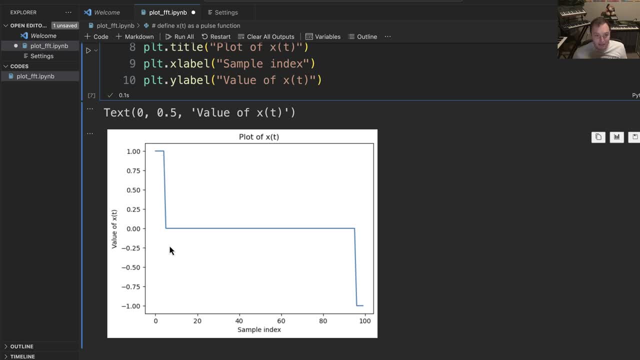 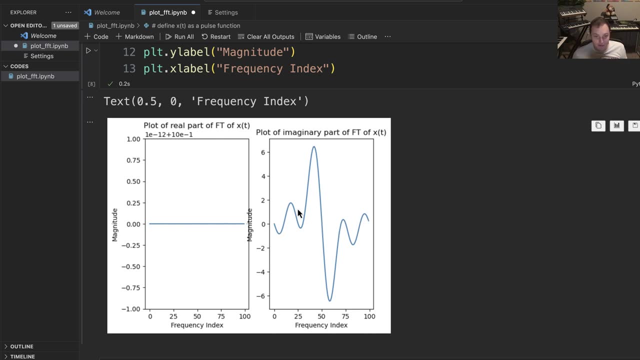 If it's a mix of both, it's going to have both components. But because this signal is completely real, we have conjugate symmetry, meaning the imaginary part, the positive part, is equal to the negative of the negative part, And then the real part is even symmetric. The one thing to 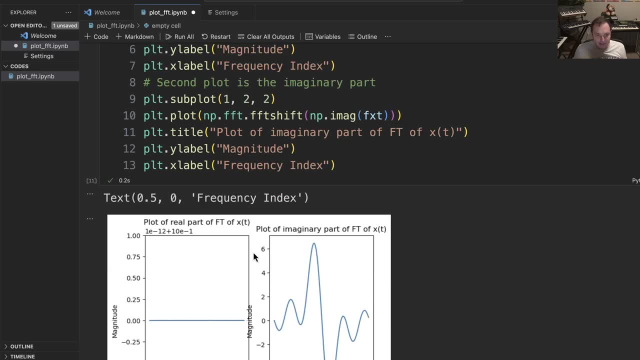 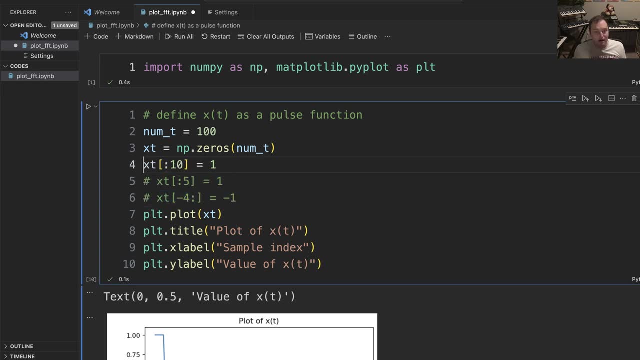 remember is that you're always plotting something that's a combination of a real and imaginary part. Now, if you want to plot this in terms of polar form instead of rectangular form, we can do that as well. So I'm going to run this back to what we had before. So we have both. 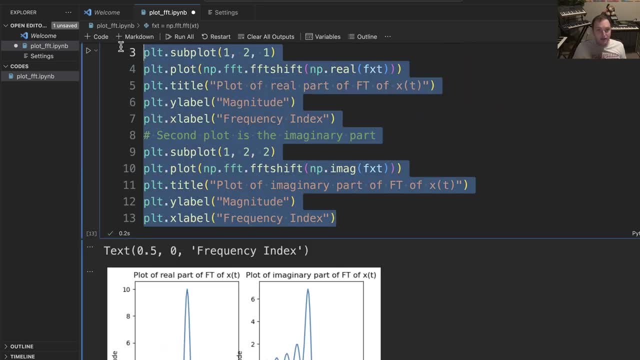 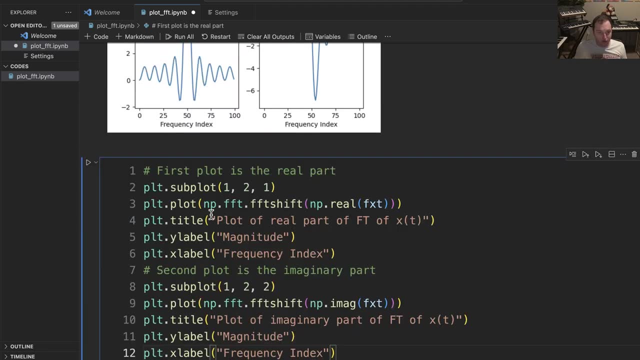 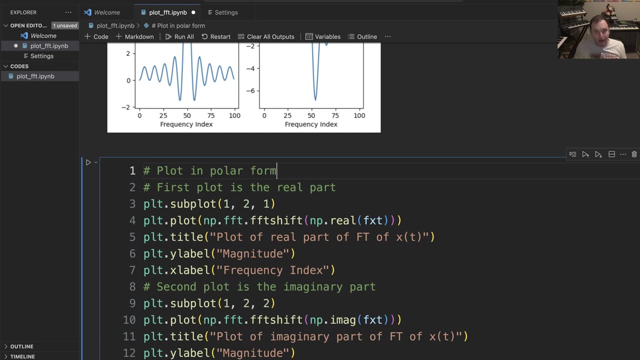 a real and an imaginary component, And what I'm going to do is copy my plot, except this time I'm going to plot it a little bit differently. So this is going to be the plot in polar form, Plot in polar form, And what we're going to see here is: